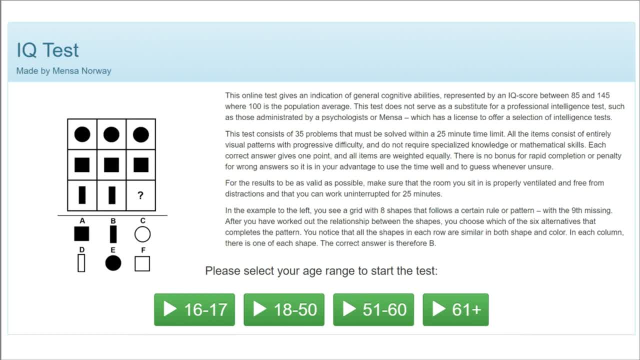 Welcome to the Puzzles and Solutions channel. Today I will be looking at the Mensa Norway IQ test. A friend sent me this IQ test some days ago and I wanted to make a video about it going through each puzzle and what solution. If you would like to take the test yourself, the link. 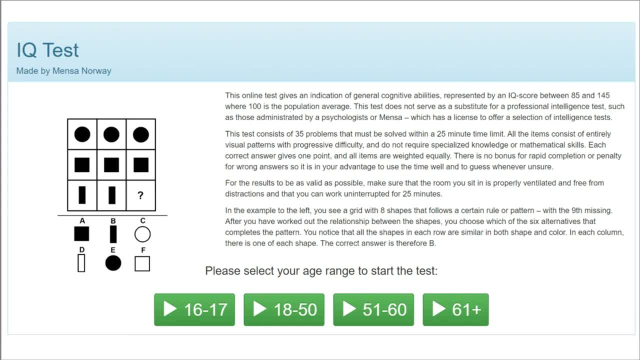 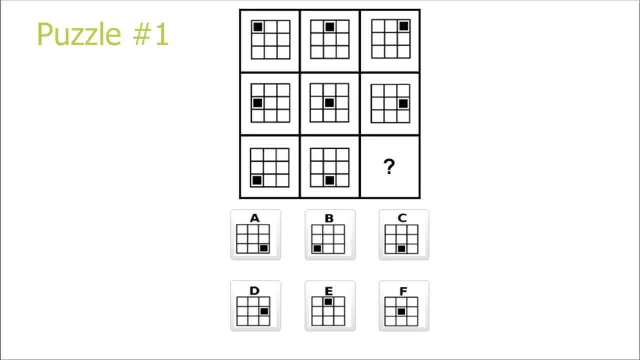 will be in the description. I also suggest that you pause the video at the higher difficulty puzzles and try solving it yourself before listening to my solution, Puzzle number one, Each picture is a 3x3 grid showing a miniature version of the IQ test itself. So, since it's the 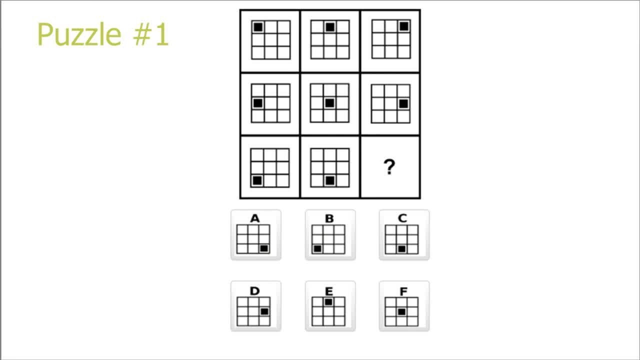 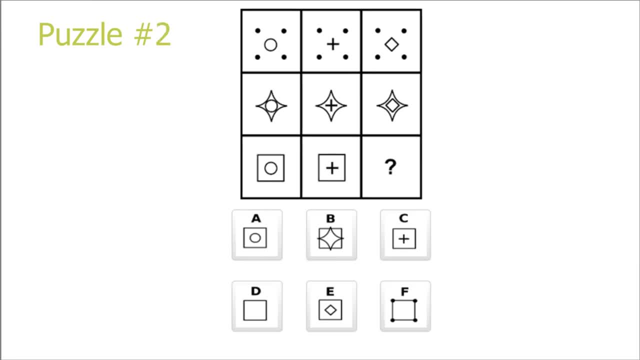 last picture to the right and the last picture downwards. we also know that the solution will have a black square in the most right and most downwards position. So the answer is A Puzzle. two: By looking from top to bottom, we see that the first column only have a circle in the middle. 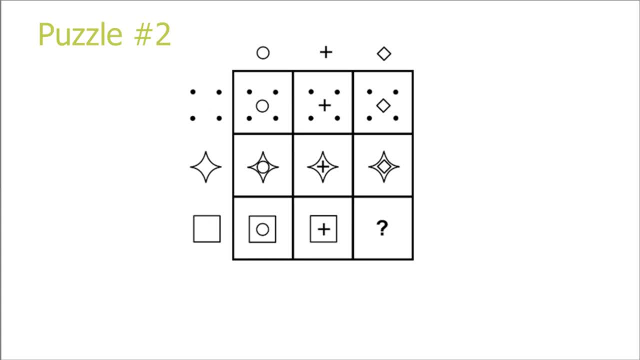 the second column only have a plus sign in the middle and the last only have the rotated square in the middle And by looking at the rows we see four dots repeating in the first row, star in the second row and square in the last row. Therefore, the picture will have a square with a rotated 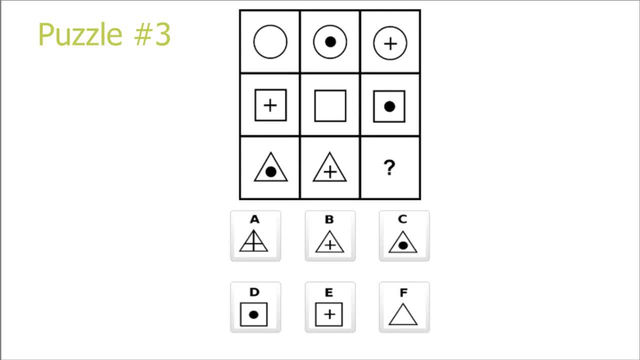 square inside from the top to the bottom, And the last picture will have a square with a fit and the correct answer is E, Puzzle three. So here we have the exact same situation, but instead it's circle, square, triangle, on the rows and on the diagonal from the top left to the bottom right. 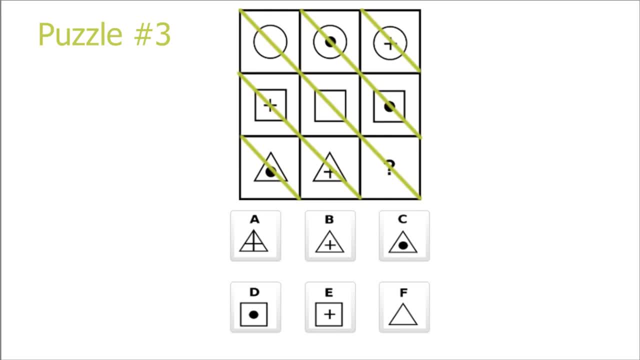 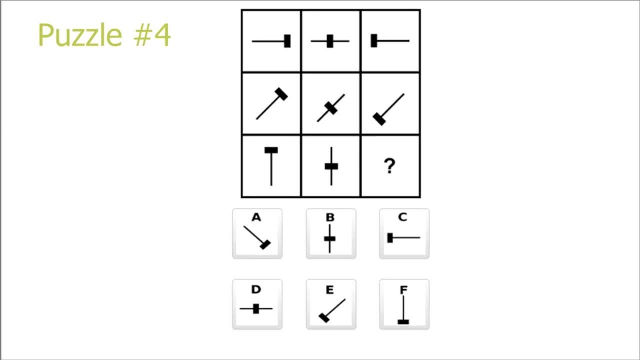 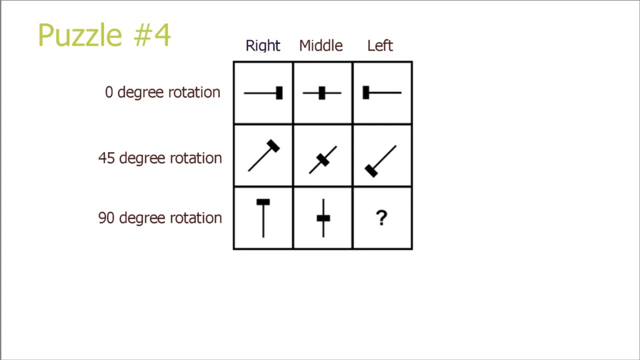 we have plus sign, dot and nothing. So our answer will be a triangle with nothing inside it, which is F Puzzle four. This puzzle is kind of similar, except it's a moving part going from column to column and a rotation going from row to row, So there is a zero degree rotation for the five. 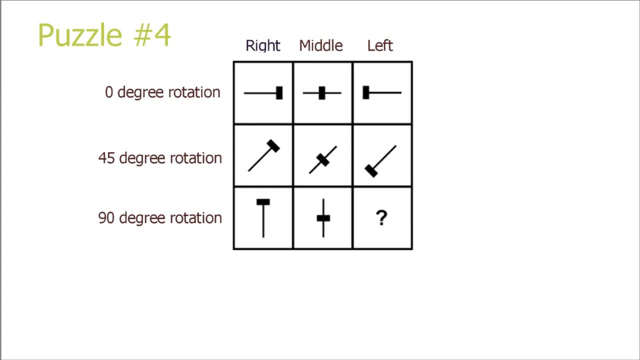 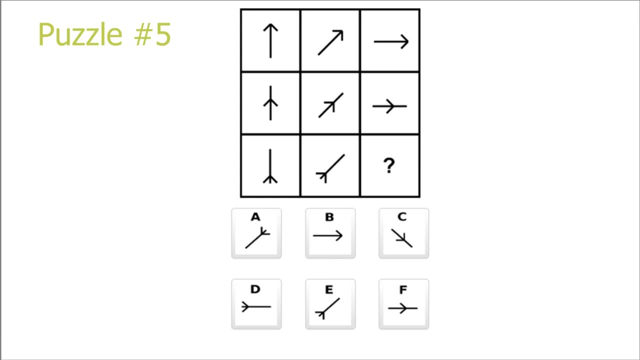 and a 90 degree rotation. So, yeah, we can either base on ourself on the row and just move the black square to the bottom, or we can take the column and rotate the picture 45 degrees And, as you can see, this is our option. F, Puzzle five. This is the exact same as the previous one, just rotation on. 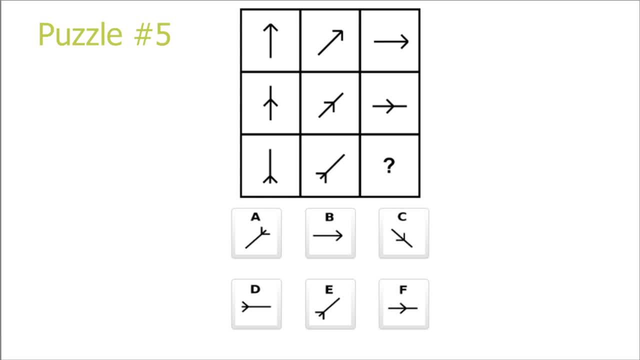 the columns and moving downwards on the rows. And again you can either rotate on rows or pull it back on the columns and we get the answer. D Puzzle six. So here we see some black squares and if we look at the top black squares we see that 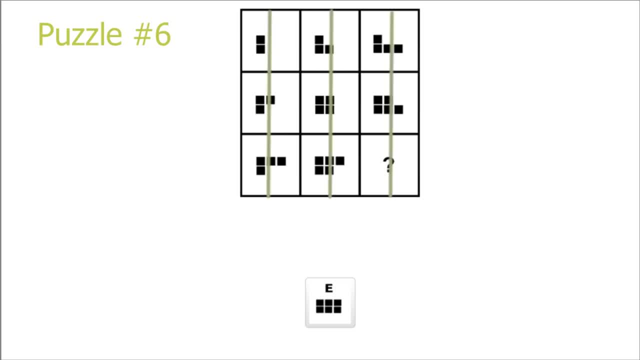 there is the same amount on every row and if we look at the bottom black squares we see that it's the same on every column. So we get that it's three on top and three on bottom and our answer is E Puzzle seven. Here we have the exact same situation for the rows and the columns and 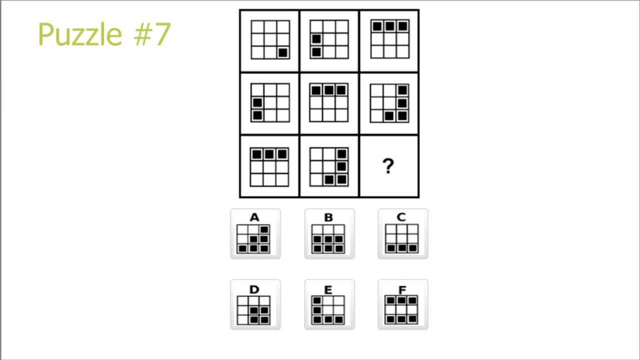 all we do is we rotate the picture 90 degrees and then we add a black square at the most clockwise position compared to the other squares. So here we take picture eight, rotate it 90 degrees and add a black square at the most clockwise position, which will be in the top left corner, and we get. 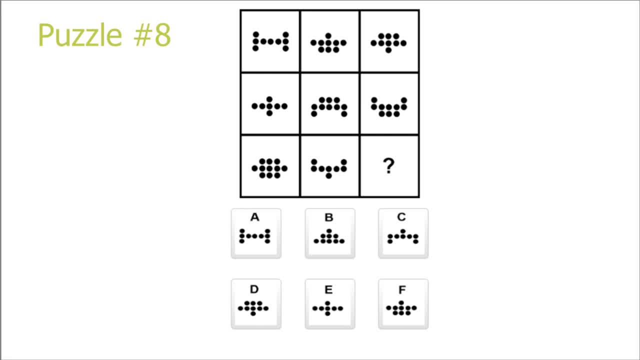 the answer E, Puzzle eight. If we look at the bottom half of the pictures, we see that in the diagonal from the top left to the bottom right, they repeat in every picture. and if we look at the top half, we see that they repeat in the diagonal from the top right to the bottom left. 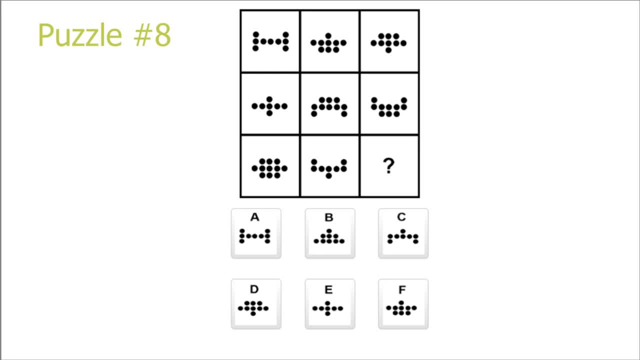 Also, the diagonal from the top right to the bottom left repeats every three diagonals. We know that it will be a dot in the middle, on the top half. This leads to answer C. We could also easily solve this by seeing that column three is just column two and then rotated 90 degrees. 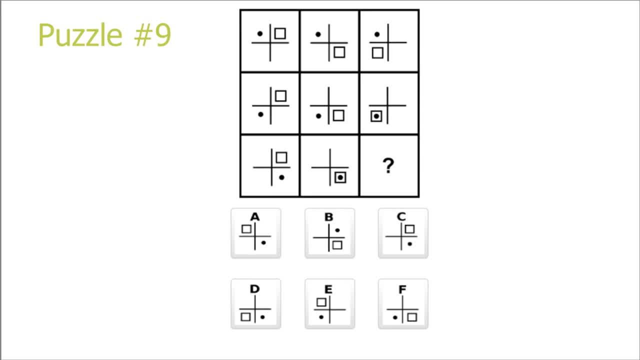 Puzzle nine. This is another row and column puzzle. We see that the black dot repeats itself on every row in the same position and for every square. we see that it repeats itself for every column. So in the last column we have a white square on the bottom left and on the last. 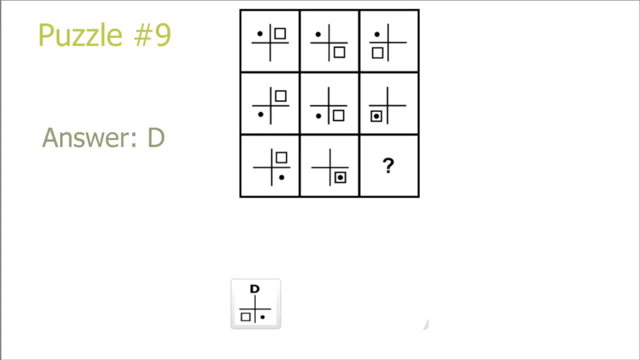 row we have a black dot on the bottom right. So we have the answer D, Puzzle ten. The easiest way to solve this puzzle is just by looking at the rows and see that each picture is the previous one, rotated 90 degrees counterclockwise. So if we take our picture eight and rotate it 90 degrees, 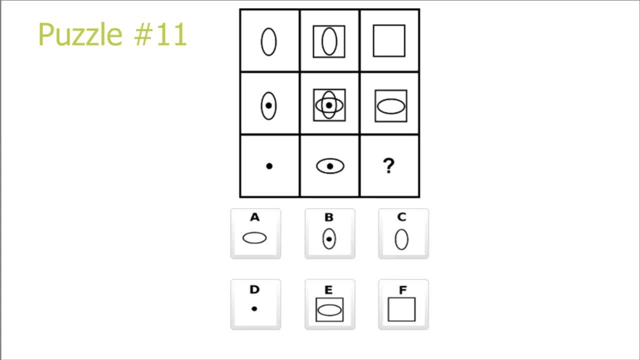 counterclockwise we get the picture D Puzzle eleven. This is a new kind of puzzle. If you look at the second row, you see that the second row is just the first row added with the second row. So if you look at the third row you see that the second row is just the first row added with the 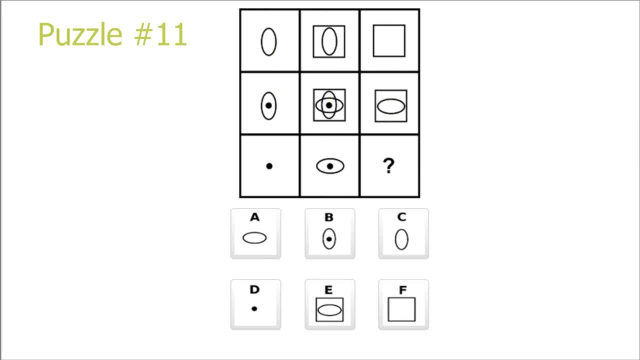 third row. Also, if you look at the columns, the second column is just the first column added together with last column. So if you look at the last row, we get that picture eight minus picture seven is picture nine. So all we have to do is remove the black dot and we get that. A is the. 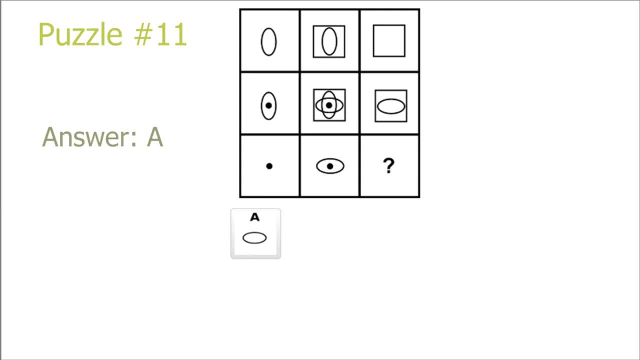 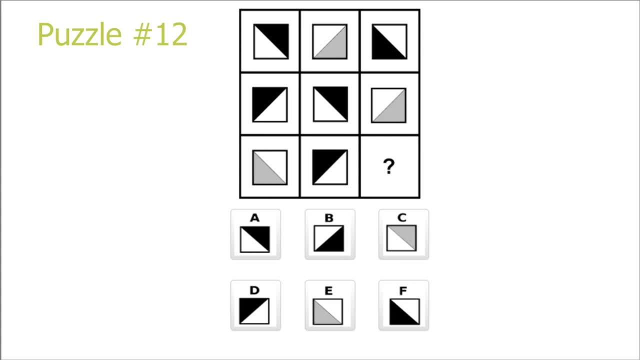 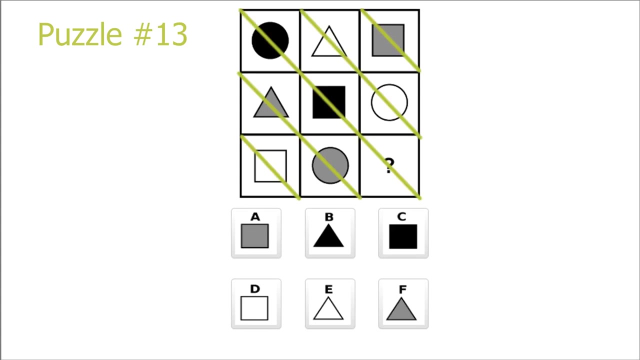 correct solution. We can do the same for the column. so we have that. picture six minus picture three equals picture A. So again the same solution, Puzzle thirteen. If we look at the diagonal from the top left to the bottom right, we see that the 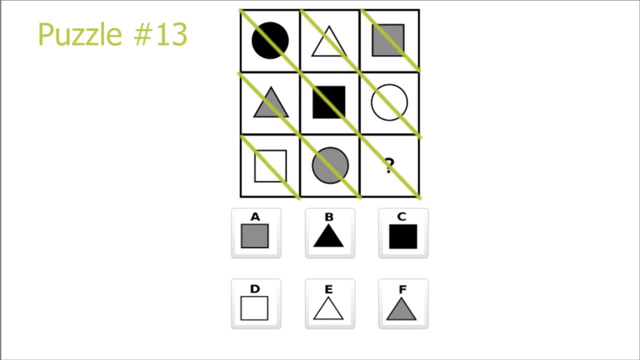 colors are repeating, So we have a black picture as our answer. Also, if we see from the top right to the bottom left diagonal, we see that the shapes are repeating and they're repeating every three diagonals, So we have, after circle comes triangles, so we have a black triangle as our answer. 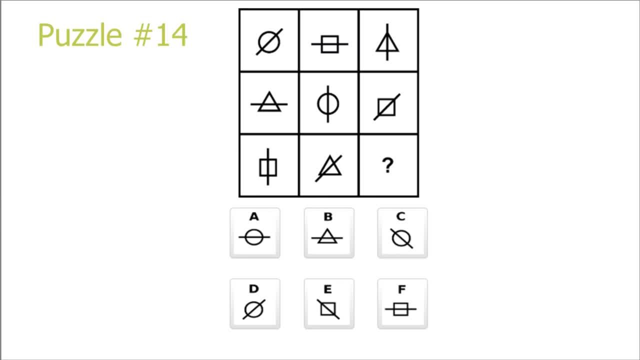 Puzzle fourteen. So here we have the same thing with the top left to the bottom right diagonal, but in this case it's the shapes. So we have a circle and if you look from the top right to the bottom left diagonal, we have that the diagonals are repeating every three diagonals And we have 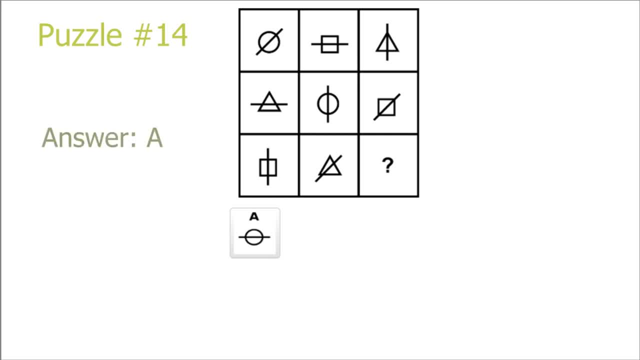 a horizontal line as our correct solution. So A is the correct answer. Puzzle fifteen: Exact same again. So we have the triangle's orientation in the top left to the bottom right corner, which leaves a triangle pointing upwards, And then we have a repetition every three diagonals going from. 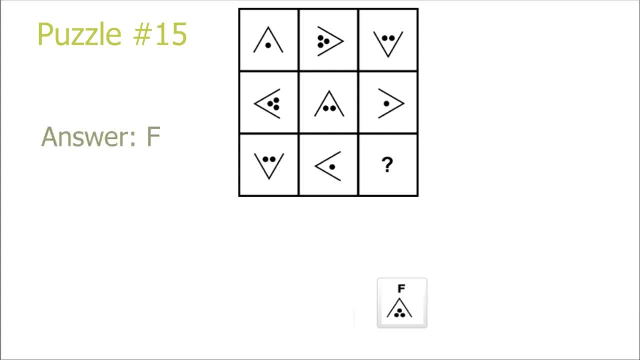 top left to bottom right, which leaves F as the correct answer. Puzzle fourteen: This puzzle is exactly the same as the previous puzzle. Instead we have that it's the color which repeats on the top left to the bottom right diagonal, And then we have these shapes which rotate ninety degrees per diagonal. So we get 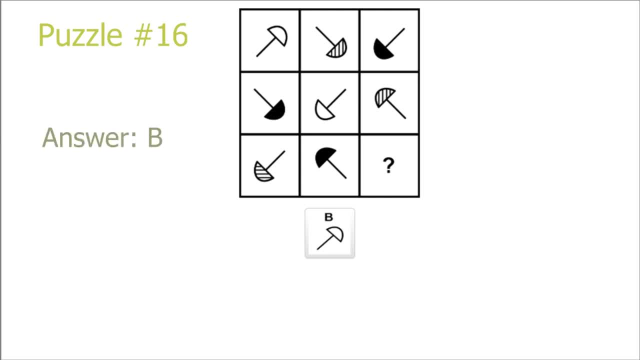 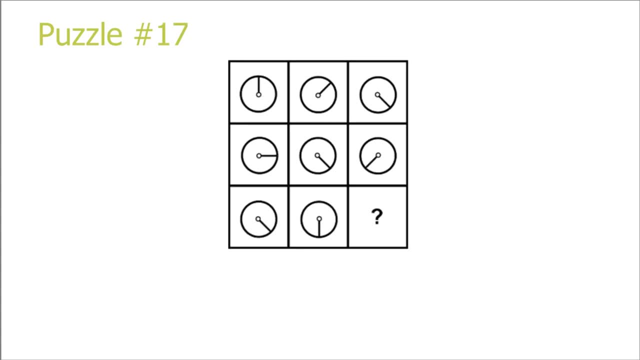 that it repeats every four diagonals and we get that. the correct answer is B, Puzzle seventeen. So this puzzle is easiest solved by just looking at the rows. So first we have a forty five degree rotation clockwise and then we have a ninety degree rotation clockwise. 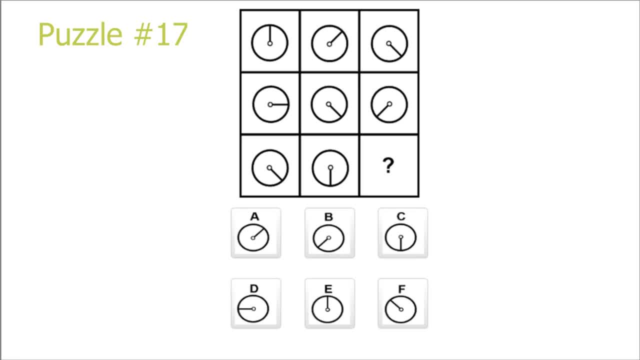 So we base ourselves on picture eight and we rotate it ninety degrees clockwise and we get picture D, Puzzle eighteen. So in this puzzle we see that there is a repetition in the columns. so we know that we shouldn't base ourselves on the columns. So we know that we shouldn't base our 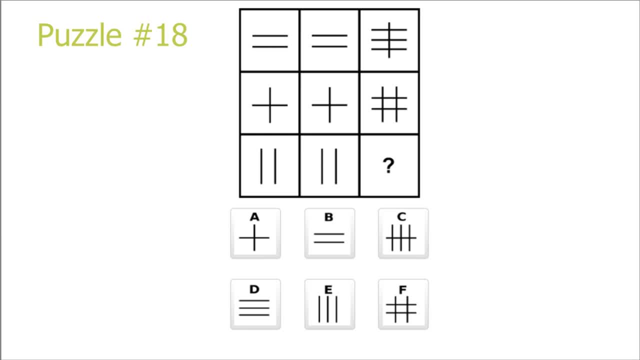 self on the columns. So we go by the rows and we see that moving down one row leads to a horizontal line transitioning into a vertical line, And this is consistent for every picture, in every row. So we know that our answer is picture eight, with one horizontal line swapped out for a vertical. 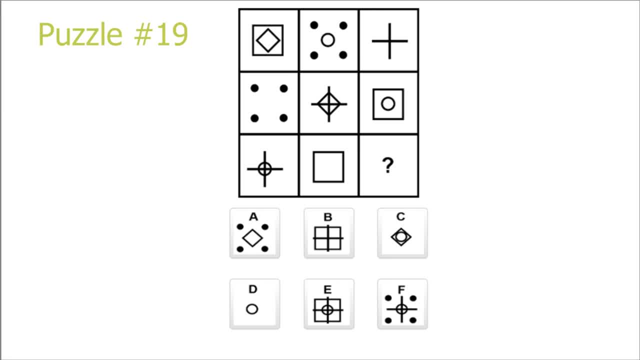 line and our answer is C. Puzzle nineteen. This is another diagonal puzzle. We see that there is a repetition of circle, rotated, square and nothing going from the top left to the bottom right diagonal Square. four dots plus sign going from the top left to the bottom right diagonal. 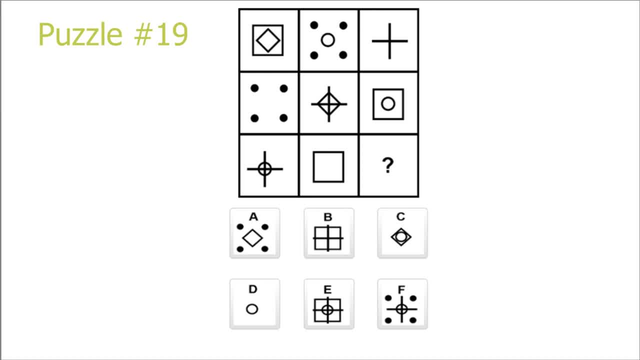 So we know our answer contains four dots and a rotated square in the center. so our answer is A Puzzle twenty. So here we have a new puzzle. It goes like this: We add two pictures and we just remove this overlapping line, and that leads to the last picture. This is consistent. 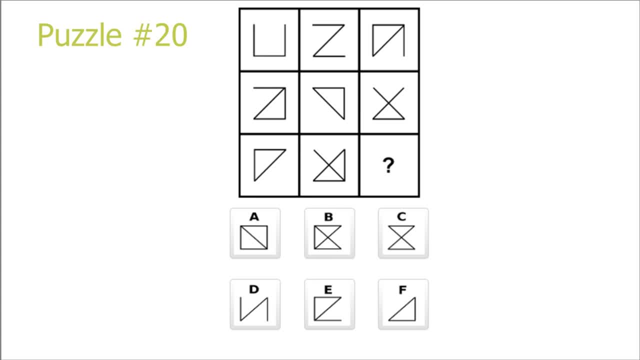 for both the columns and the rows. So we just add together picture seven and picture eight and we get a square which has a line going from the top left to the bottom right corner, which is A Puzzle 21.. So here we have the exact same situation as the previous puzzle, so we can just 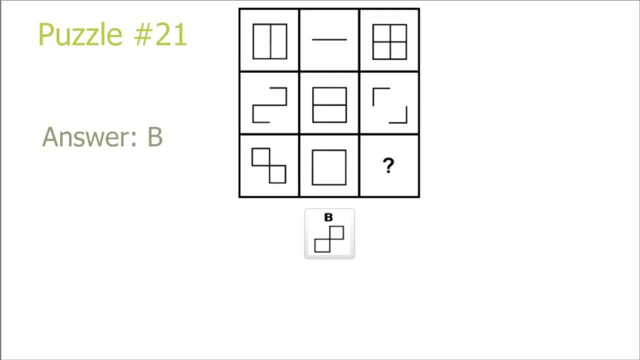 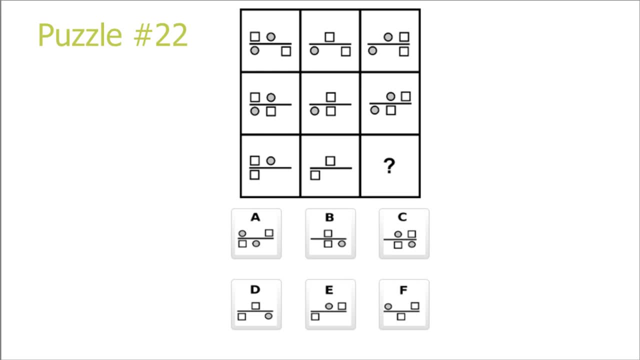 add picture 7 and picture 8 and we get that B is the correct solution, Puzzle 22.. Here we have a row and column puzzle. If you look at the bottom of the picture we see that it repeats on the rows, and if you look at the top of the picture we see that it repeats on the columns. So we have our 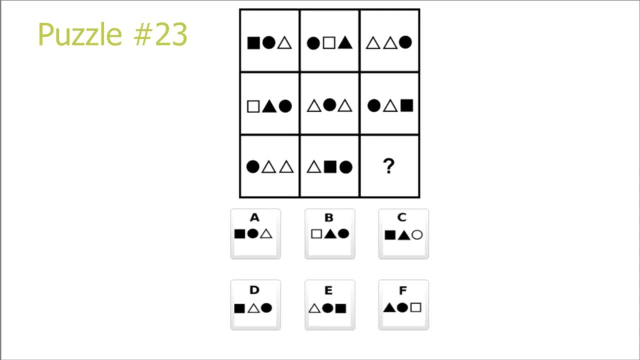 answer E, Puzzle 23.. This is a diagonal from the top right to the bottom left puzzle and by looking at the main diagonal we see that the picture itself is also rotated, like the shapes inside it is rotated. so we base ourselves on picture 4 and we rotated it one to the left, which results in: 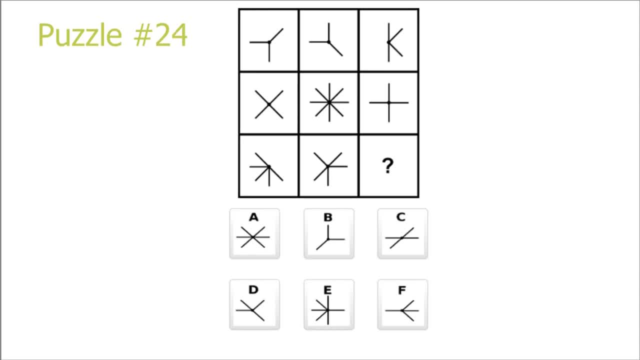 picture F, Puzzle 24.. Another addition and removing the overlapping line puzzle. and we get that the correct answer is F Puzzle 25.. This is a new union In this unique puzzle which we haven't solved yet. we see that the overlaps between row 1 and row 2 is 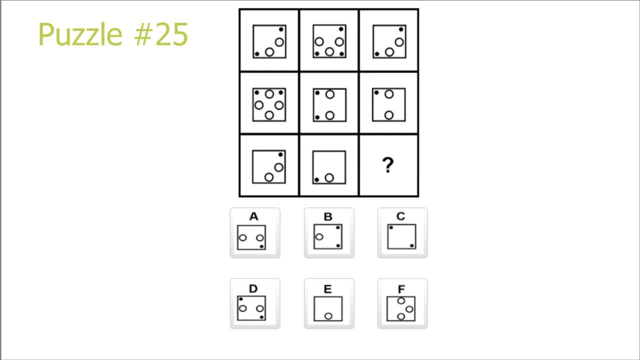 row 3, or that the overlaps of column 1 and column 2 is column 3.. So we can either base ourselves on picture 3 and picture 6 and see what they have in common, or picture 7 and picture 8 and see what. 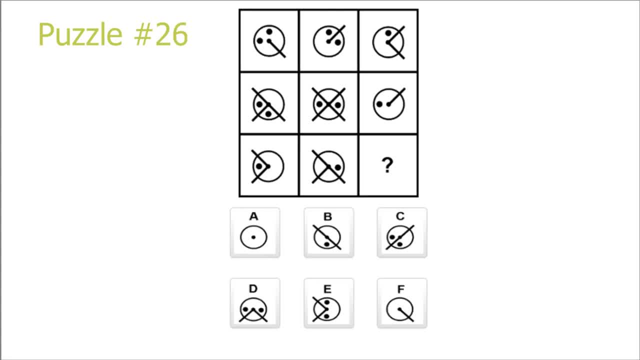 they have in common and they both lead to our solution, E Puzzle 26.. If we look at the rows in this picture, we see that the last picture is just the intersection of the rows and the columns. So black dots in picture 1 and 2 and the addition of the lines in picture 1 and 2, and if there is 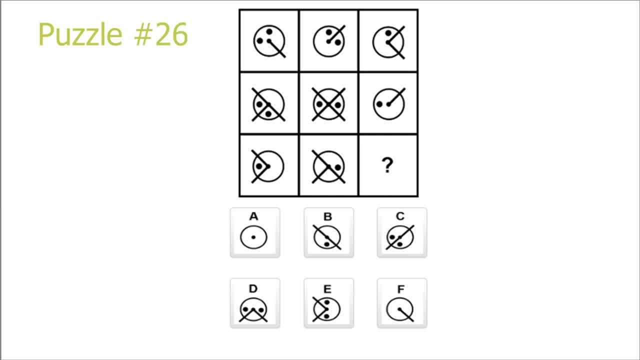 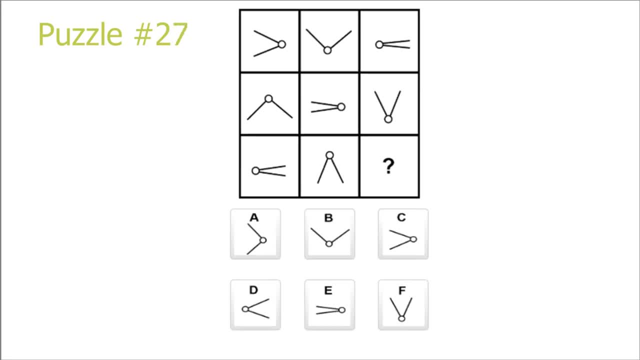 overlaps of the lines. they cancel each other out. We can also go by columns with some different rules and we get picture F for both solutions, Puzzle 27.. Here we see there is a rotation on the rows by 90 degrees clockwise and there is a change of shape in every rotation. so we get 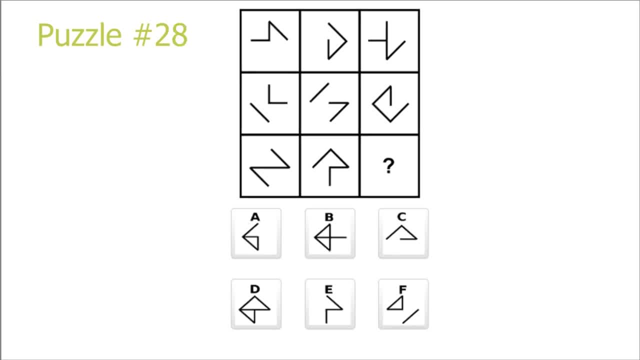 that A is the correct solution. Puzzle 28.. Another addition and canceling puzzle: If we add picture 7 and 8, we get that A is the correct solution. So now we start on the six last puzzles, which are also the hardest ones. If we look at rows or columns here, we see: 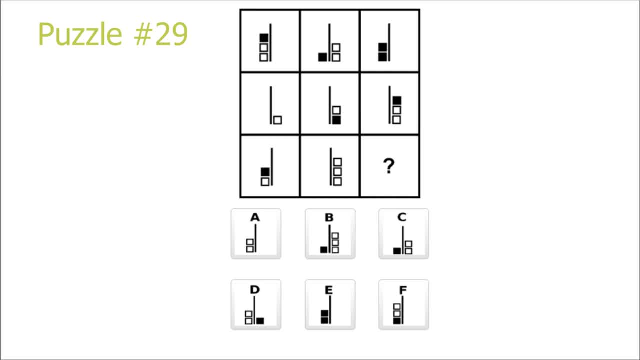 that our last picture is just our first picture and our second picture added together. If there are similar squares on both sides, they cancel each other out. So if we look at our first row, we see that both white squares cancel each other out and the black squares just add together. 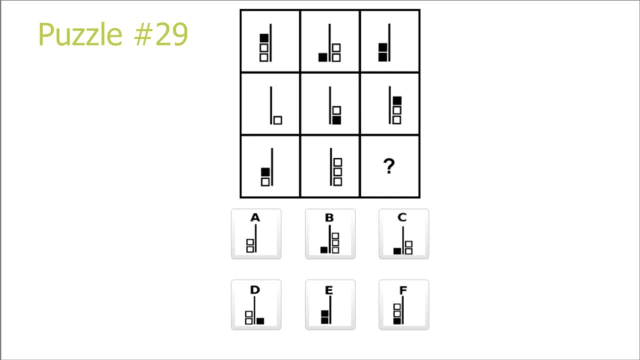 To have two black squares and if you look at the second column, we have that the black squares cancel each other out and the white squares just stack on top of each other. So we can base ourselves on rows or columns, and if you look at the last row, we see that white is cancelled out. 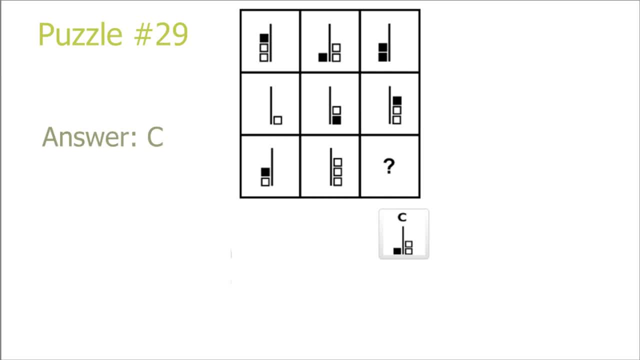 on the right side. So we have two whites on the right side and one black on the left side and we have the answer C, Puzzle 30.. So here we have an addition puzzle and we have to figure out how the answer is. So, for example, if we add a dot with a dot, what does that result in? and if you look at 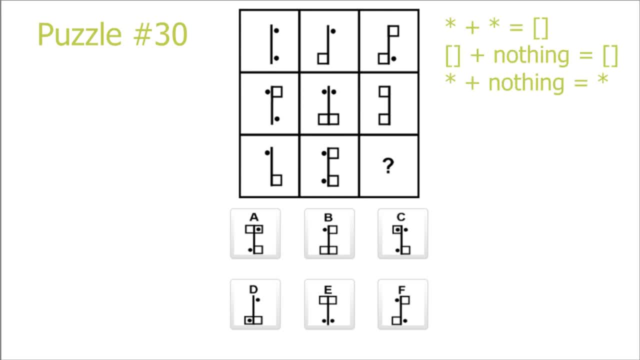 the first row we can do these three rules: Dot plus dot equals square, Square plus nothing equals square, Dot plus nothing equals dot. And by looking at the second row we see a new rule which is square plus dot, and we get that square plus dot equals nothing. And for the final rule we have to look. 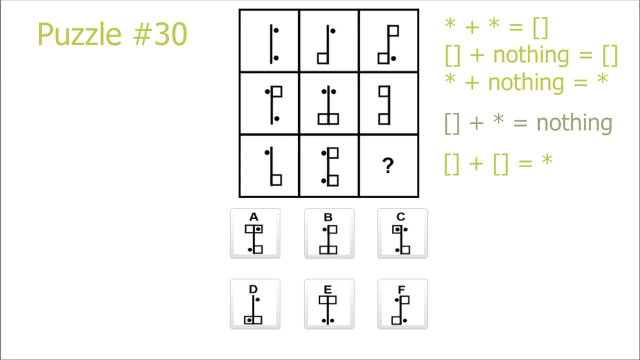 at the second column and we get that square plus square equals dot. We can use this rule for both the last row or the last column to deduce our picture. So we see that there is a square in the top left corner, a square in the top right corner, a dot in the bottom left. 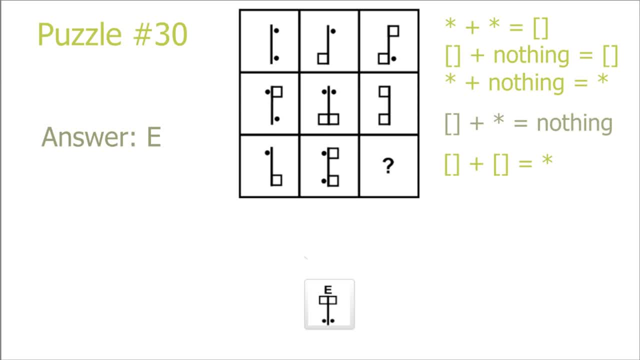 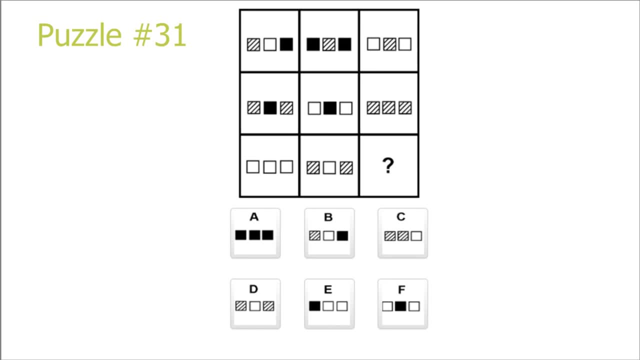 corner and a dot in the bottom right corner. So E is the correct answer. Puzzle 31.. So I found some patterns in this puzzle, but I didn't figure out the correct solution and I'll go over why A, B or D is the correct answer. So if you look from the top, 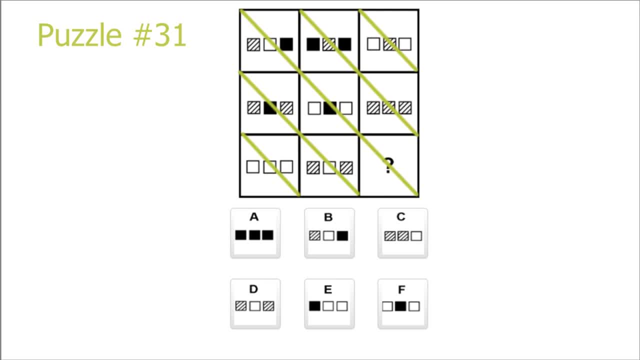 left to the bottom right diagonal. there is an inversion of our stripes into white and white into stripes in our main diagonal from top right to bottom left. To see this more clear, I'll redraw the picture in terms of just the rows and columns, and we get this picture So we can clearly see moving from row one to 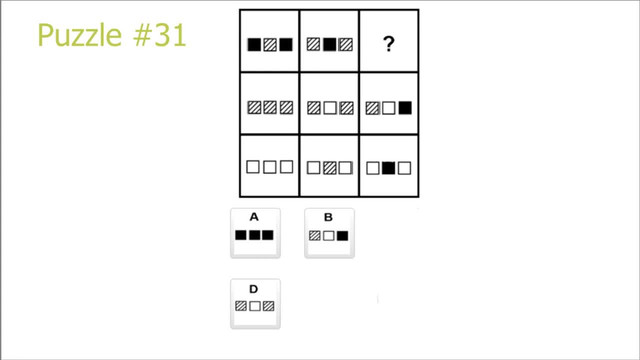 row two, there is no change in the white or striped, and moving from row two to row three leads an inversion of the stripes and whites, leading the whites to become stripes and stripes to become whites. And also going from column one to column two or column two to column three, the colors of the most left and most right squared. 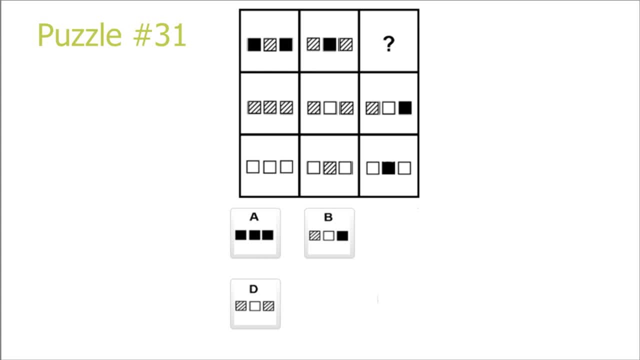 is kept the same when they are striped or white, And from column one to column two there is an inversion of the middle square, going from white to stripe or stripe to white, and the middle square from column two to column three it's kept the same color. So from all this we can deduce that our 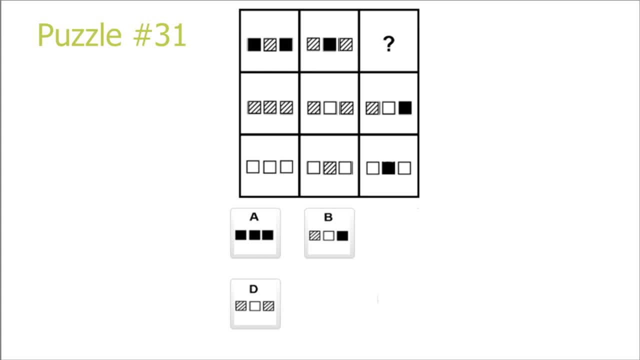 answer has striped, white, striped pattern. There might be black squares which hide over these patterns, So all we need to do is to find a pattern for the black squares. The only one I found was that two, one, three repeating, but it's so arbitrary that I 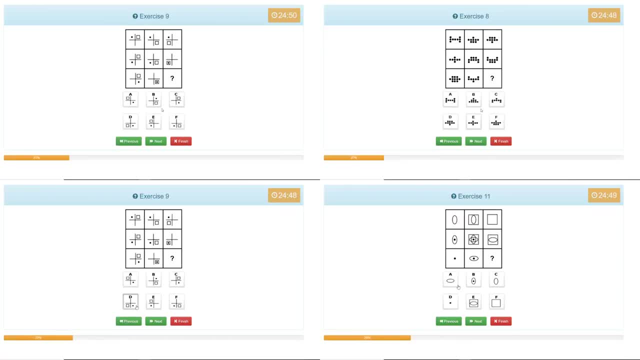 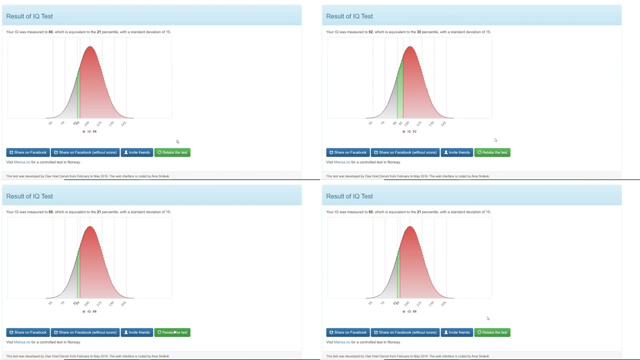 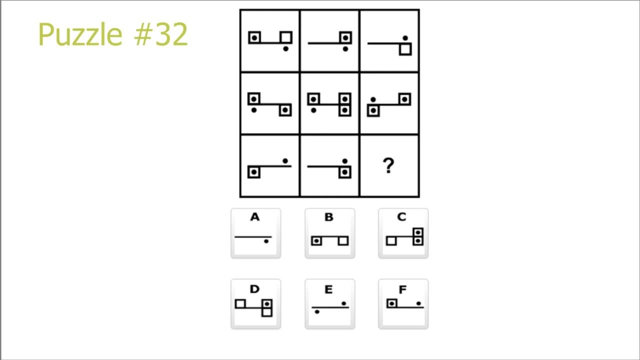 don't really call it a pattern. Now, to prove that B is in fact the correct answer, I will retake the test four times where I vote B and three other answers in the others, and I will get a hierarchy When I vote B. so therefore, B is correct. Puzzle 32. so this is way easier than the last puzzle. All we need to. 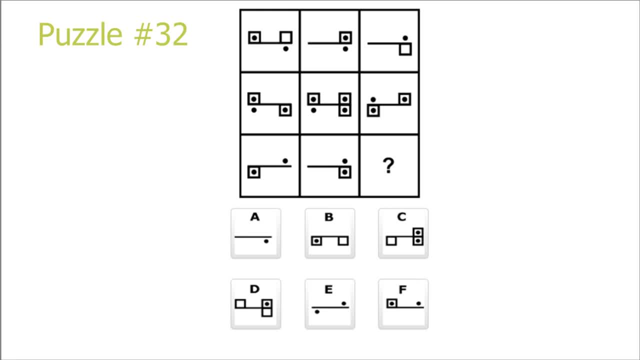 do is we look at the first or second row or first and second column, and then we see the similarities in the last row or column and then we just switch the sides so bottom becomes top and top becomes bottom. So if we compare picture seven and picture eight, we have that they have a black dot on the. 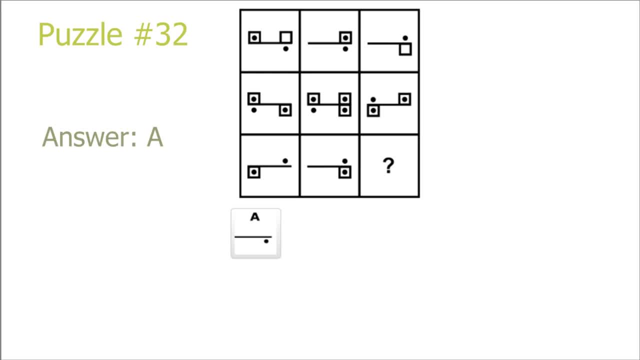 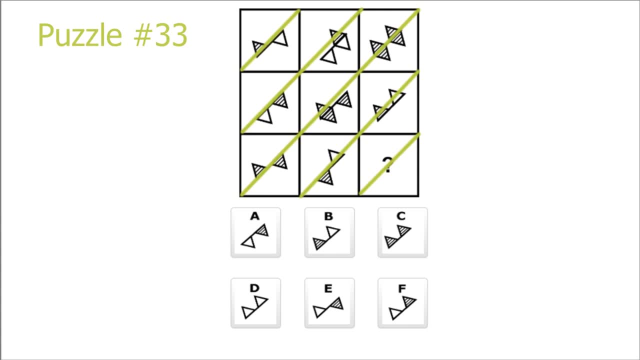 top right in common. So we take this, we swap sides And we get picture A is correct. Puzzle 33: this is another diagonal puzzle from top right to bottom left. If we compare the first row and the second row in this diagonal, we see that the right side is always changed and the rules are that. 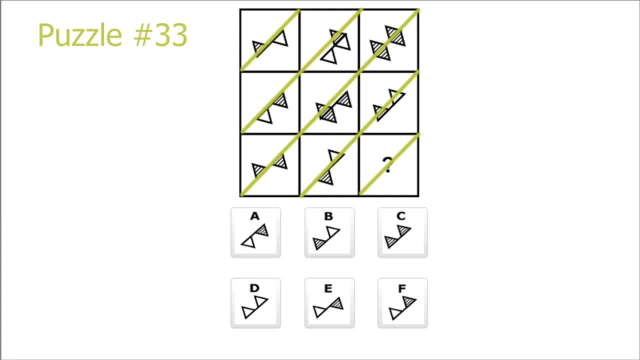 the top right is prioritized to be swapped with the bottom right, But if there is no top right, then the bottom right is swapped for the top right. And if we look at the relationship between the second and the third row, we have that the bottom left square is prioritized to swap over to the top side, but if there are none, 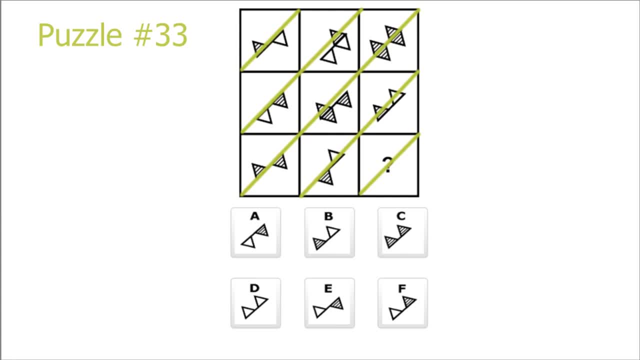 then the top left is swapped out for the bottom right. Now, in order to see this, I changed the picture so that it becomes a diagonal and column puzzle, And we see that the pattern holds true. So if we take picture six and then we swap over bottom left triangle, we have that E is 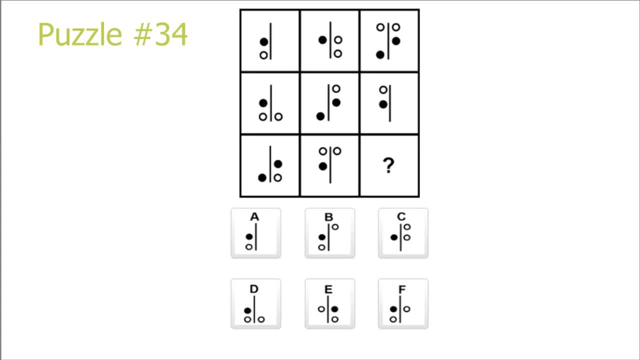 the correct solution. Puzzle 34. so this is another puzzle. going from the diagonal from top right to bottom left, We see that there is a repetition of the black dots and where they are placed. So yeah, we can deduce that there is a black dot in the. 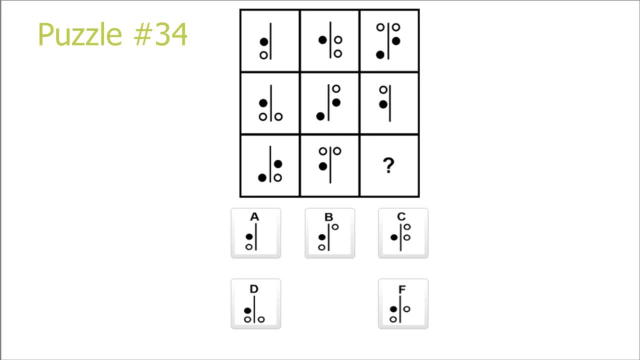 left middle. And now for the white dots. there are two ways to deduce the answer. Either we can see that there is a pattern, the pattern in the rows, where the white covers all the possible spaces in each row, with the black squares covering over the white squares. 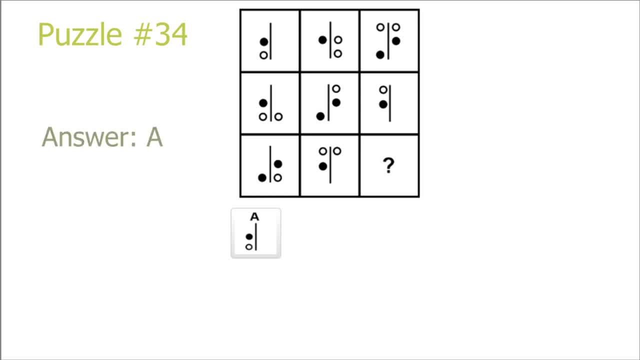 Which results in the answer A. Or we can see that from the diagonal, from top right to bottom left, the white squares are rotated clockwise one position. So we take our picture four and then we rotate the whites clockwise once and we get picture A again. Puzzle 35: I found this puzzle. 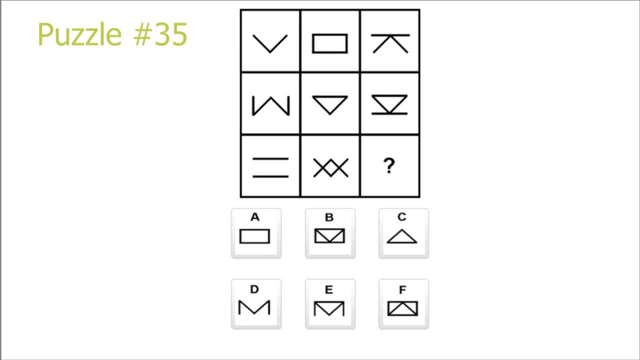 surprisingly easy compared to the other hard ones. All you need to see is that in the diagonals there are repeating patterns. So if we look from the top left to the bottom right diagonal, we have that there is there is this V shape which repeats on our main diagonal. And if you look at the top right to the